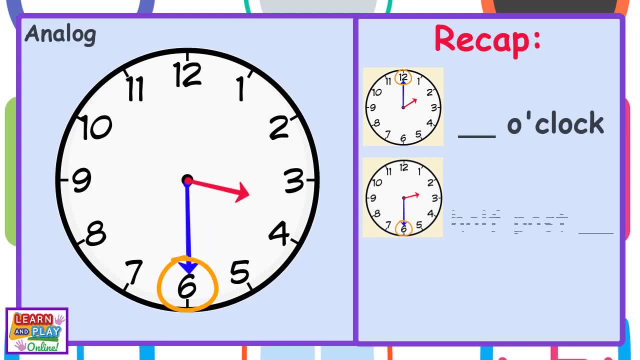 When the minute hand is pointing at the number 12, we say it is something o'clock. When the minute hand is pointing at the number 6, we say it is half past something. And lastly, when the minute hand is pointing at the number 3, we say it is a quarter past something. 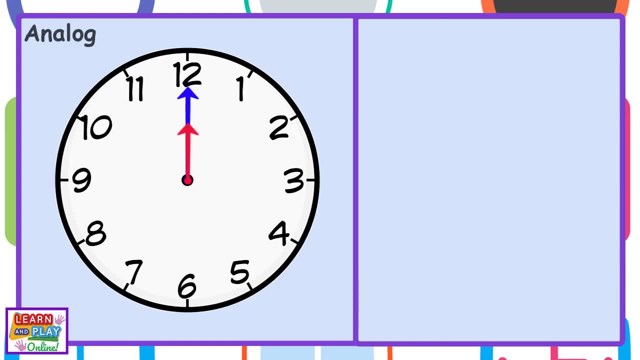 The time on the clock face now says 12 o'clock. Now watch what happens when the minute hand travels. The minute hand travels three quarters of a way around the clock face. As you can see, the minute hand is now pointing at the number 9.. 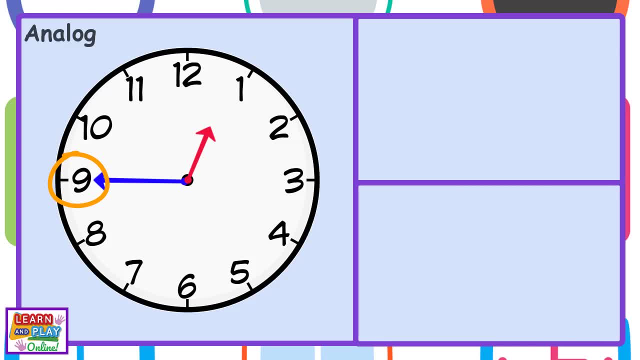 When the minute hand is pointing at the number 9 on an analogue clock, we say it is quarter 2, because there is only a quarter of an hour left until we reach the next hour. If you look at the hour hand, it is quarter 2.. 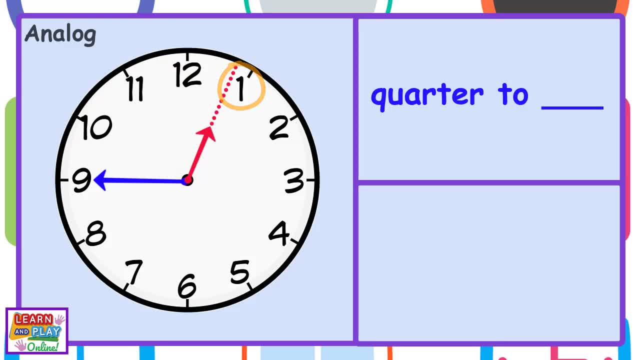 If you look at the hour hand, it is quarter 2.. It is almost at the number 1.. This means that it is a quarter to 1, because there is a quarter of an hour left until it is 1 o'clock. 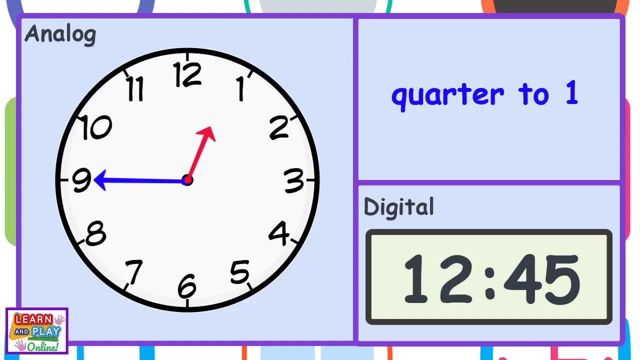 On a digital clock, it would read 12.45, because we are still in the 12th hour And when the minute hand is pointing at the number 9,, it means that 45 minutes has passed the hour, which also means that we are still in the 12th hour. 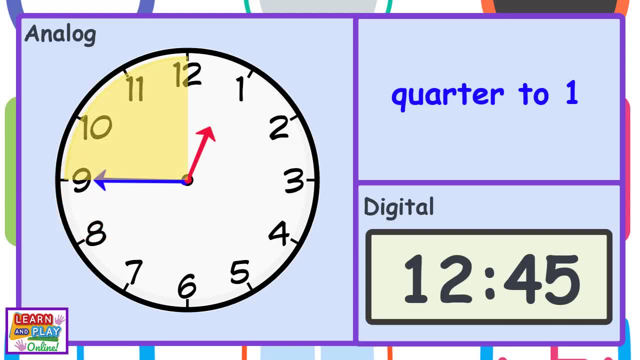 This also means that there is only a quarter of an hour left until the next hour. Now that you have learned how to read quarter 2 times, let's practice reading the times on the clock coming up. The minute hand is pointing at the number 9, so it has to be quarter 2 something. 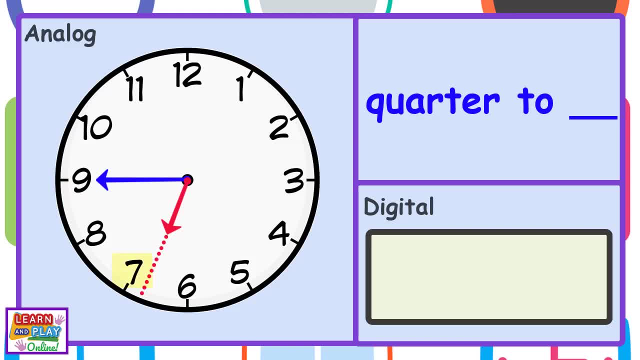 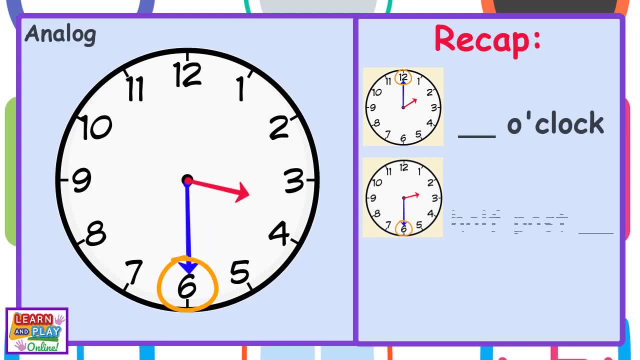 When the minute hand is pointing at the number 12, we say it is something o'clock. When the minute hand is pointing at the number 6, we say it is half past something. And lastly, when the minute hand is pointing at the number 3, we say it is a quarter past something. 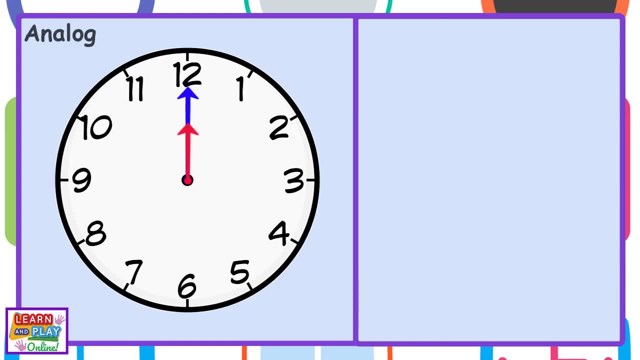 The time on the clock face now says 12 o'clock. Now watch what happens when the minute hand travels. The minute hand travels three quarters of a way around the clock face. As you can see, the minute hand is now pointing at the number 9.. 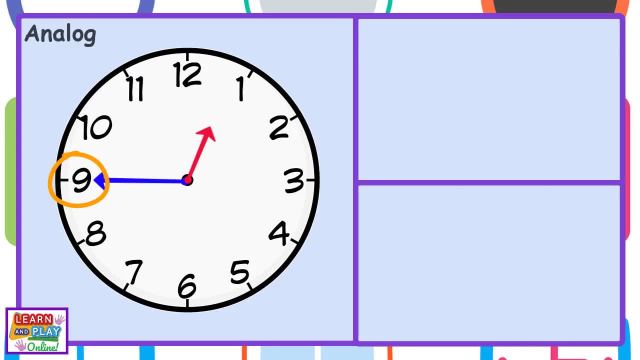 When the minute hand is pointing at the number 9 on an analogue clock we say it is quarter 2, because there is only a quarter of an hour left until we reach the next hour. If you look at the hour hand, the minute hand is almost at the number 1.. 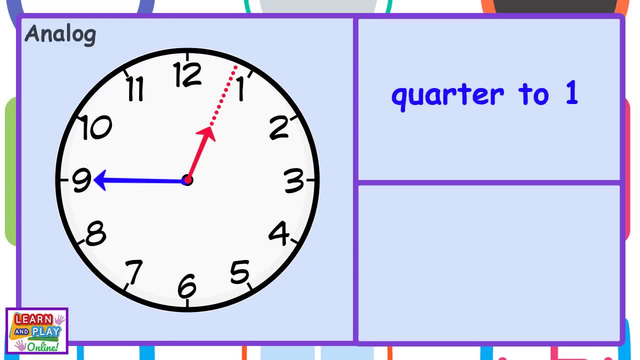 This means that it is a quarter to 1, because there is a quarter of an hour left until it is 1 o'clock. On a digital clock, it would read 12.45,, because we are still in the 12th hour. 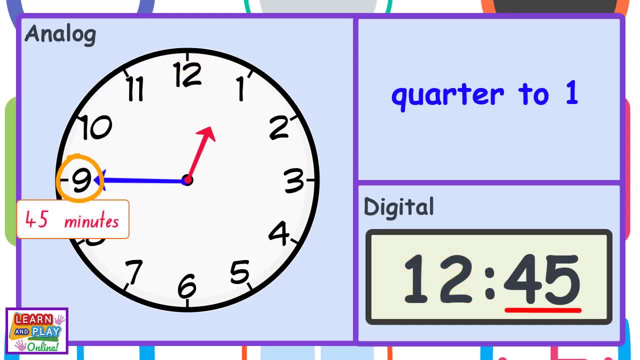 And when the minute hand is pointing at the number 9, it means that 45 minutes has passed the hour. it means that 45 minutes has passed the hour. it means that 45 minutes has passed the hour and this also means there is only a quarter of an hour left until the next hour. 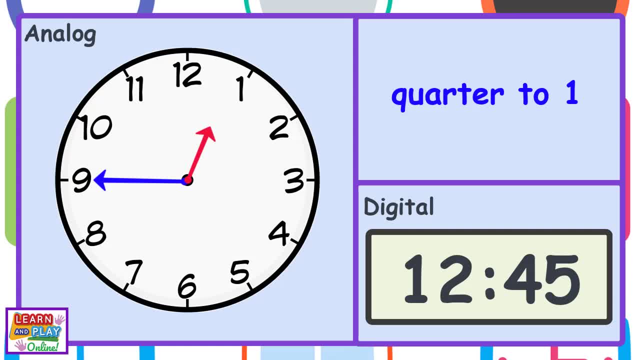 Now that you have learned how to read a quarter 2 times, let's practice reading the times on the clock coming up. The minute hand is also pointing at the number 9, so it has to be quarter 2 something. So it has to be quarter 2 acceleration. 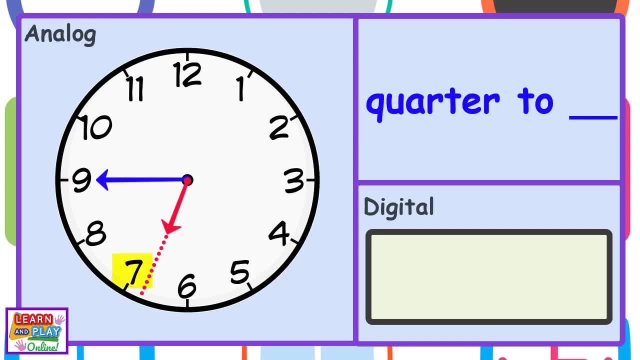 The hour hand is almost at the number 7.. So it has to be quarter 2 something. so that means it is quarter to seven or 645, because, remember, the hour hand is telling us we are still in the sixth hour. the minute hand is pointing at the 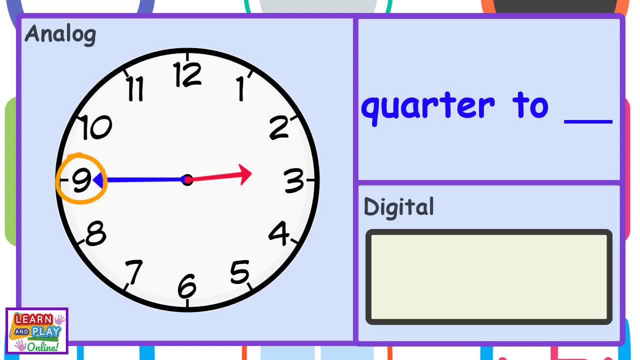 number nine, so it must be quarter to something. the hour hand is almost at the number three, so it is quarter to three or 245. the minute hand is pointing at the number nine, so it must be quarter to something. the hour hand is almost at the number 11, so 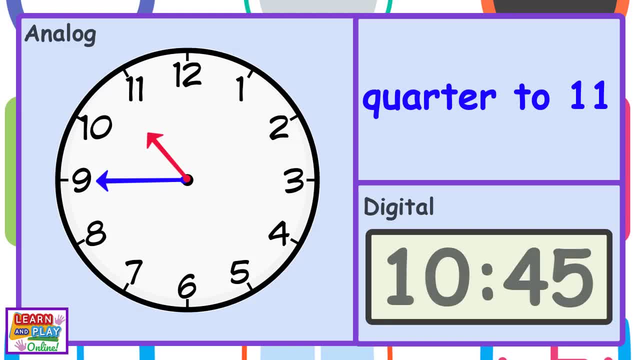 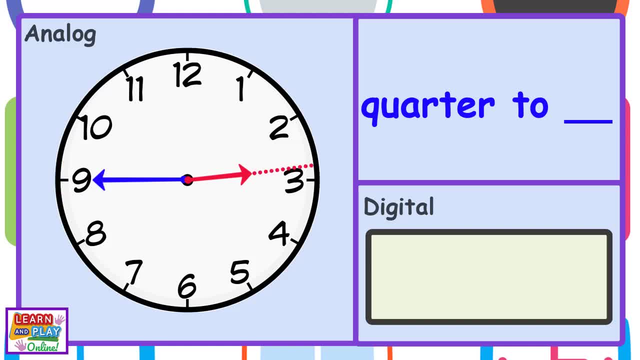 The minute hand is pointing at the number 9, so it must be quarter 2 something. The minute hand is pointing at the number 9,, so it must be quarter 2 something. The hour hand is almost at the number 3, so it is quarter to 3, or 2.45. 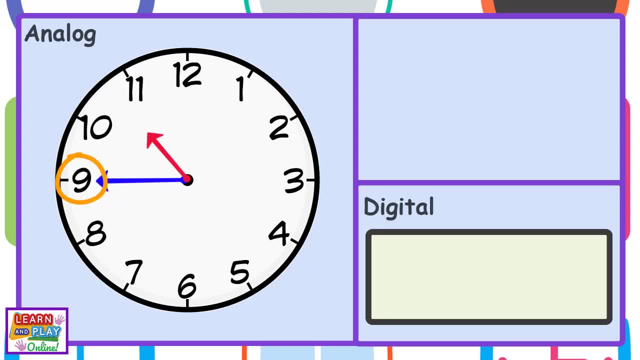 The minute is pointing at the number 9,, so it must be quarter to something. The hour hand is almost at the number 11,, so it's quarter to 11, or 10.45.. The minute hand is pointing at the number. 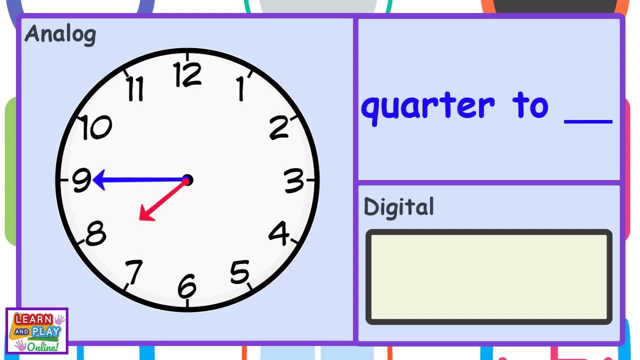 9,, so it's quarter to something. So it's quarter to 11,, or 10.45.. nine, so it must be quarter to something. the hour hand is almost at the number eight, so it is quarter to eight or seven forty five. 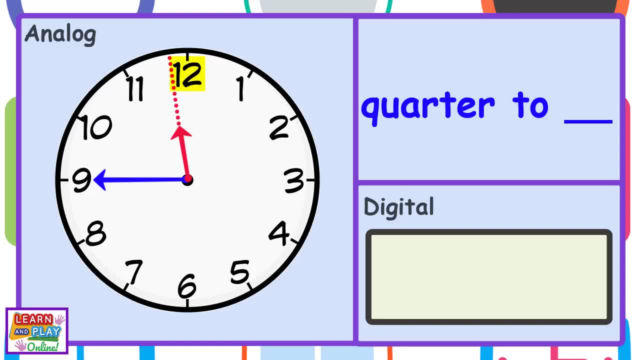